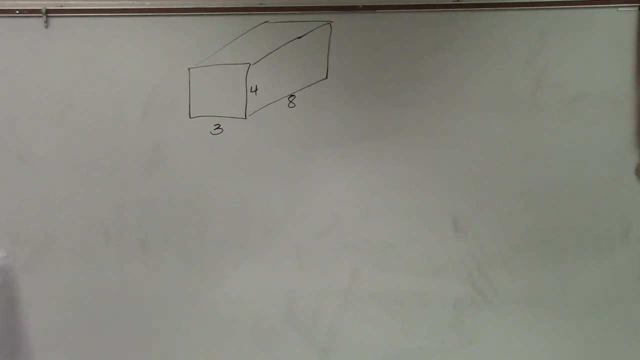 All right. so what I'm going to show you guys how to do is find the lateral surface area. If you guys look at this rectangular prism, you guys can see that there are a total of six sides. all right, And what we talked about was being able to determine which the sides are, which. 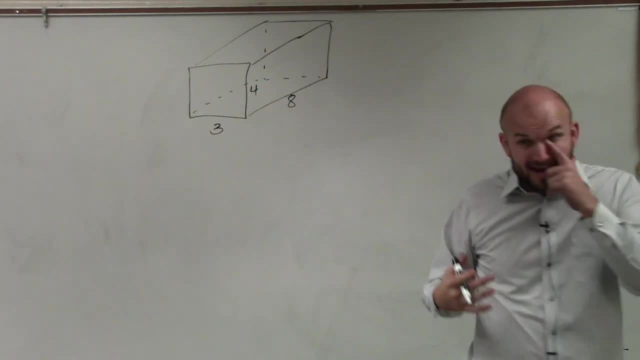 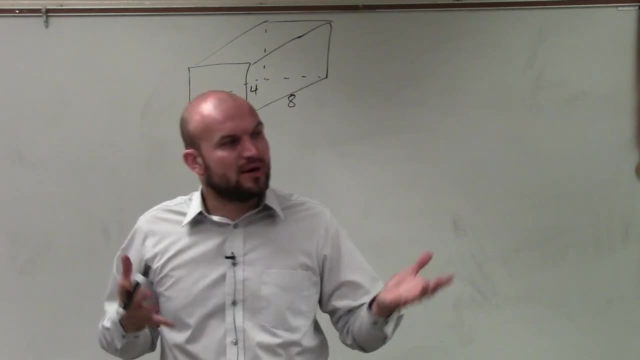 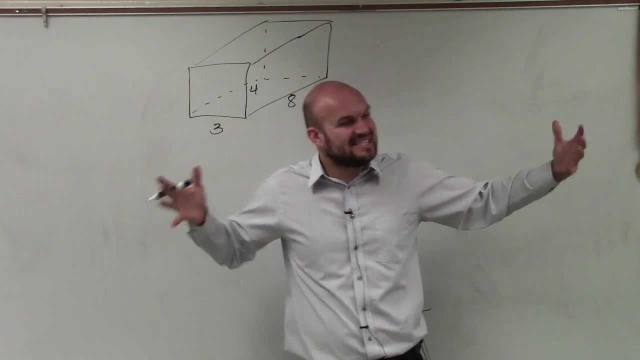 the base, the top, the left side, the right side, the front and the back, And it doesn't really matter. It doesn't really matter how you want to label them, but what I wanted you guys to understand from our examples that we did was that opposite ends of a rectangle prism have exactly 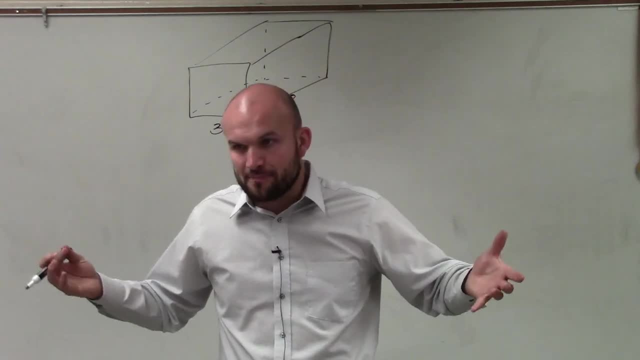 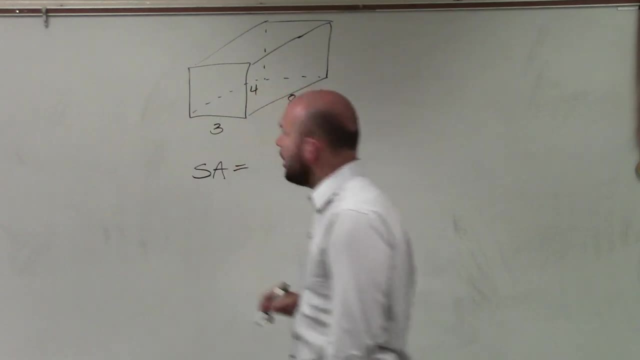 the same dimensions and exactly the same area, So we don't need to do something more often than we already have to. So to find the surface area, all I'm going to do is find the areas of the front and the back and then multiply it by two. So I'll say two times, three times four. That represents 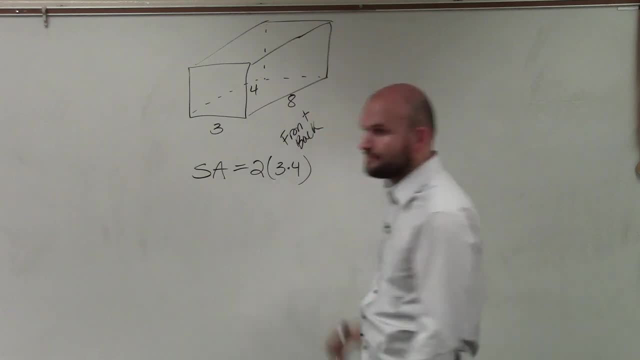 the lateral surface area. So what I'm going to do is find the areas of the front and the back and then multiply it by two. So I'll say two times three times four. That represents the front, the area of the front and the back. I'm sorry I didn't do two. Oh, because there's two. 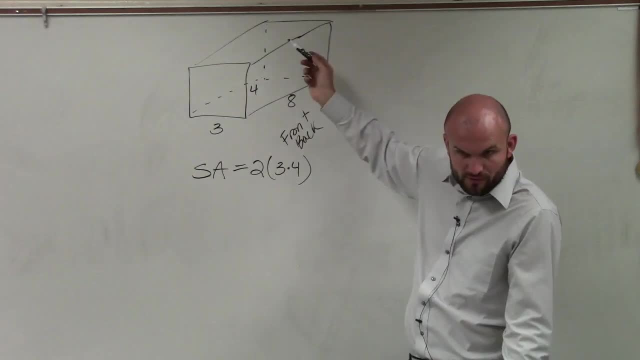 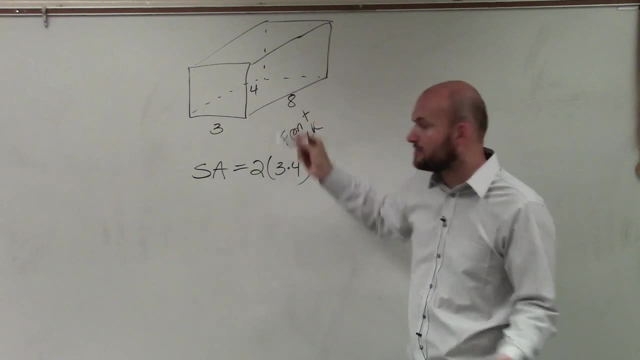 of them. Here's your front side, here's the back side, and there's two of them. They have the same area, They have the same dimensions, right? If this is a rectangular prism, if that's four, that's four. If that's three, that's three. Then we add that to two. 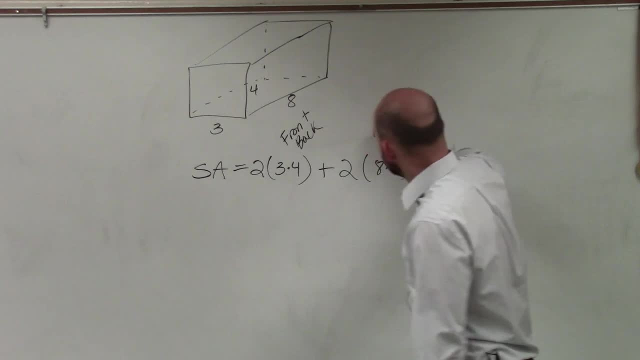 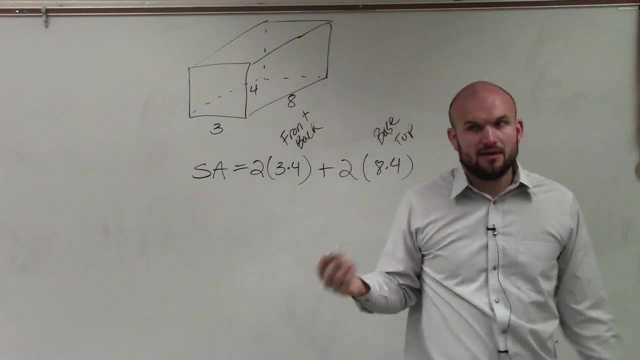 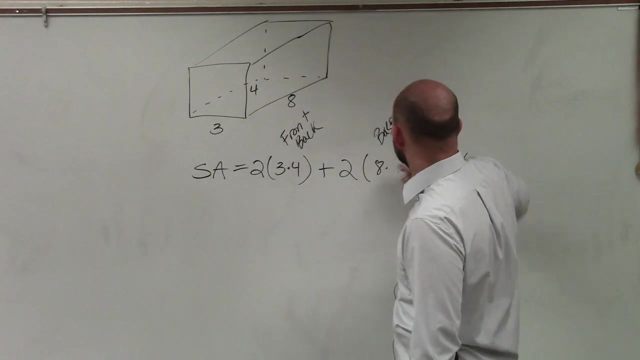 and then we'll do eight times four, which represents the area of the base and the top. Here's the base and here's the top side. Then I can add that to two times- I'm sorry, Three times eight. That was three times eight- And then this will be eight times four, which represents 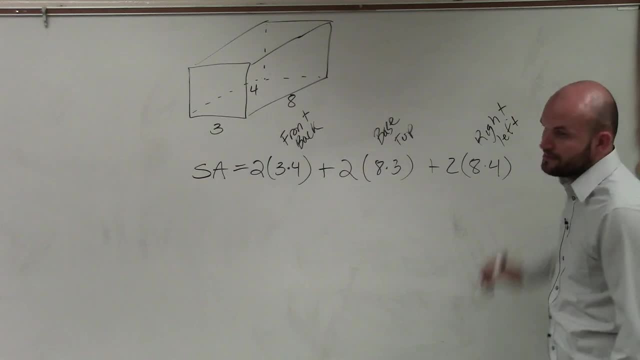 the area of the right side and the left side. So if you guys can just find the areas of three sides and then you multiply them by two, now what I can go ahead and do. you can go back around that way please.